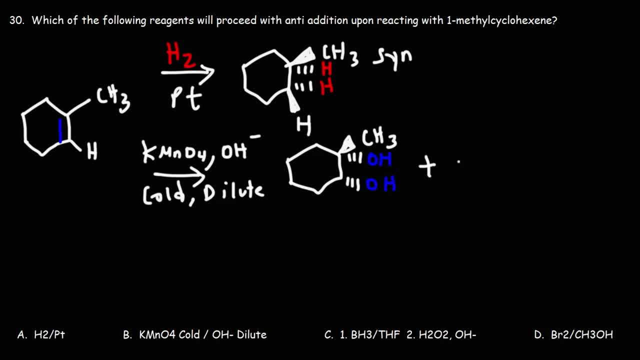 And we can also get the enantiomer as well, But this is a syn-addition reaction. Now for the next one. we have hydroboration, in the first step, BH3THF, And in the second step, oxidation. We have hydrogen peroxide. 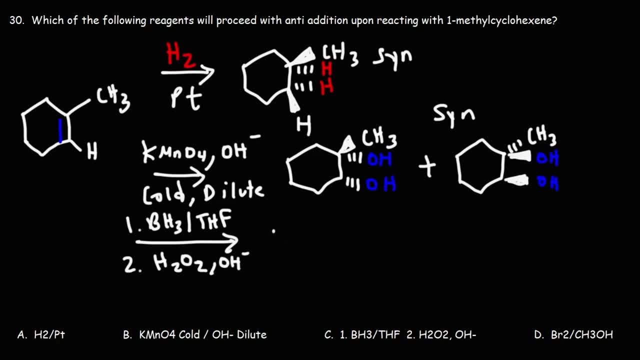 And hydroxide. So this reaction will proceed with antimarkovnikov regiochemistry, But the two things that will be added is a hydrogen and an OH group. By the way, here's the other hydrogen For those of you who are wondering. 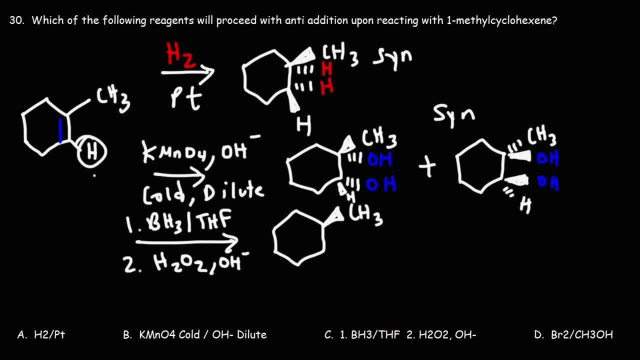 Here it is. That is the original white hydrogen. Now I'm going to highlight the two groups that are added in red. This reaction proceeds with syn-addition. The OH group is going to go on the less substituted secondary carbon of the double bond. 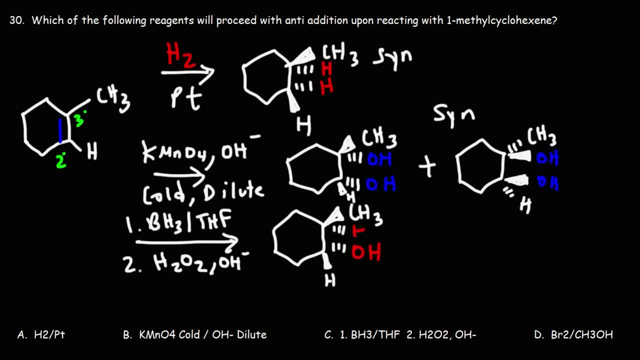 The hydrogen will go on the more substituted carbon of the double bond, That is the tertiary carbon, But it proceeds with syn-addition. Now we're also going to get the enantiomer as well. So that's the end result of the hydroboration oxidation reaction. 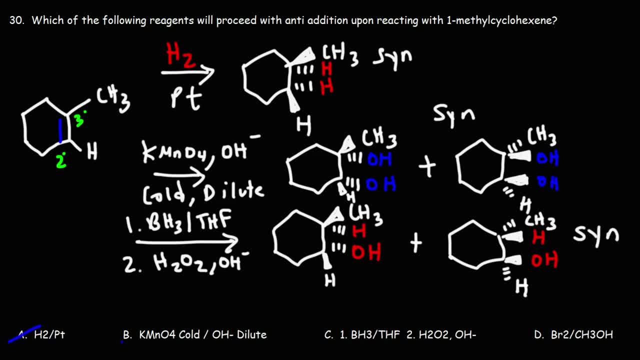 It's a syn-addition reaction, So we can eliminate answer choices A, B and C. The correct answer is going to be answer choice D. When we add Br2 with methanol, This reaction will proceed with markovnikov regiochemistry. 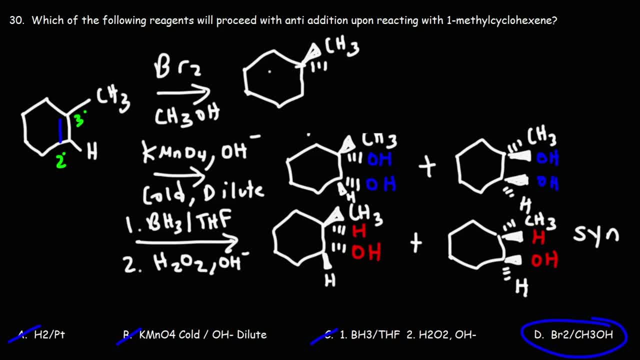 The nucleophilic ether group. That's going to go on the tertiary carbon, The more substituted carbon, Whereas the bromine will go on the less substituted secondary carbon. So when you see bromine and methanol, We're going to add one bromine atom.